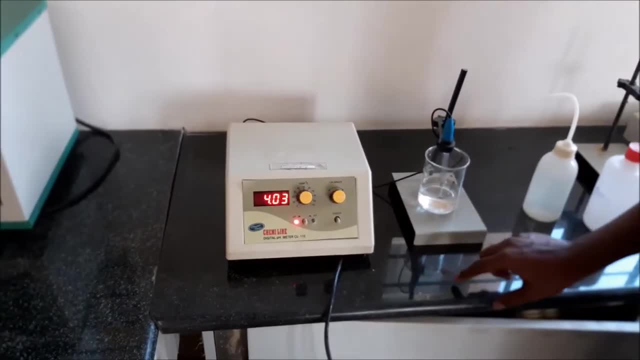 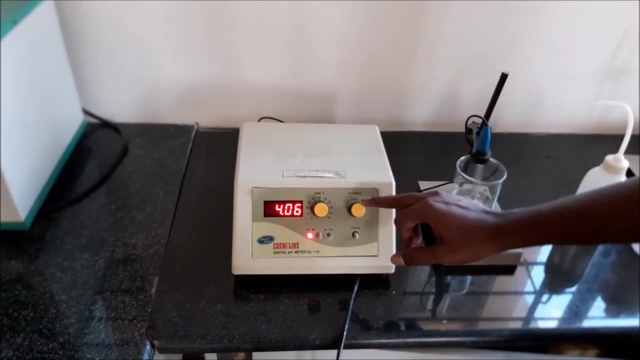 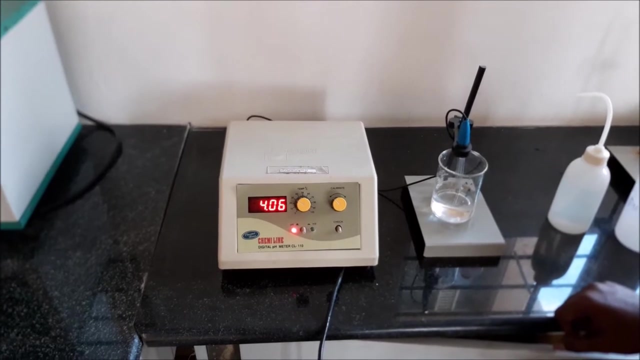 and then if you check, if you can just see the value is almost nearer to 4. but we can readjust and recalibrate it again so it's almost nearer to the 4. so the calibration of the instrument to the value of 4 is complete. 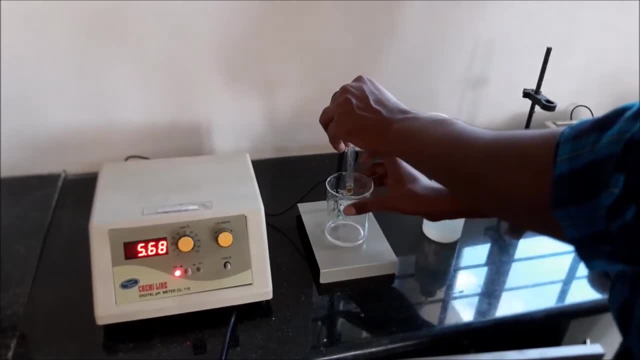 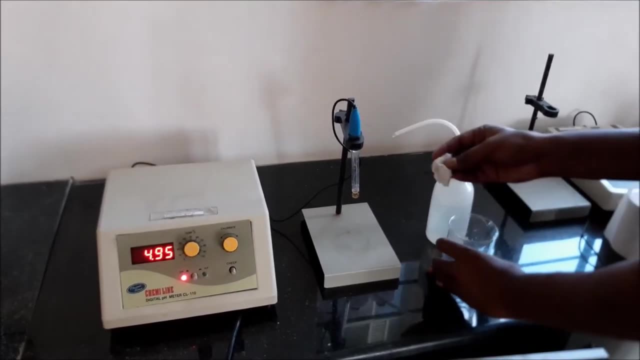 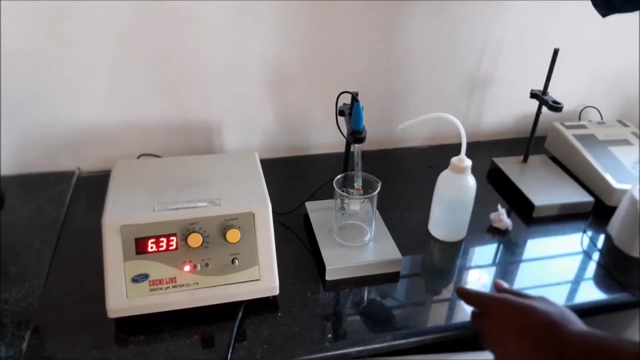 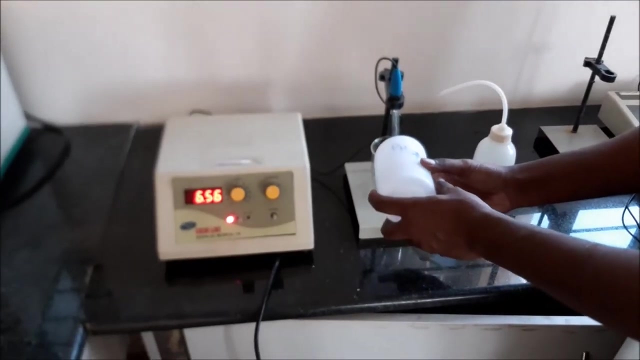 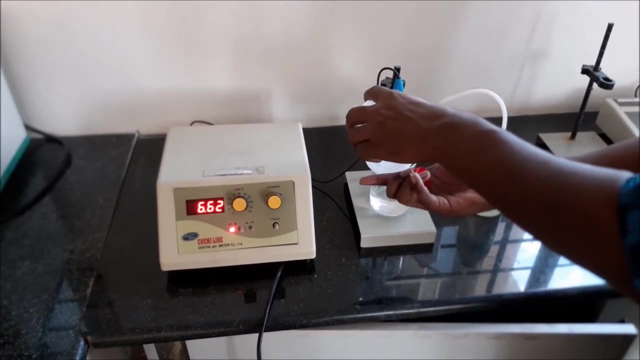 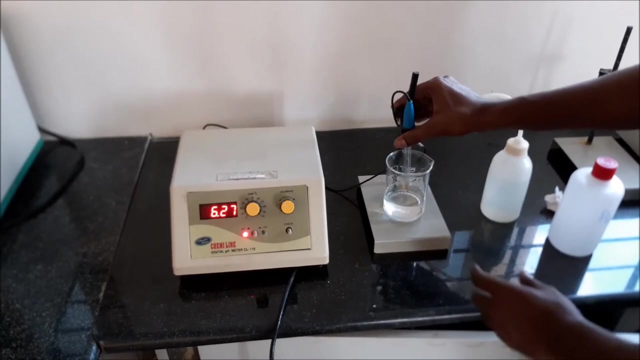 every time the instrument is cleaned with distilled water and the electrode is wiped with tissue paper, then the instrument is ready for next set of calibration. now the buffer solution for calibration of ph value equal to 7 is taken in the beaker and then the electrode is immersed into the buffer solution. 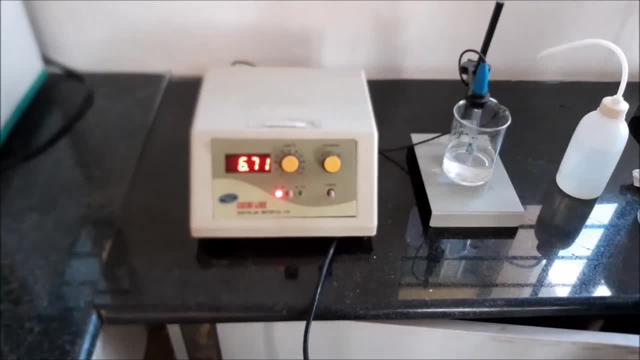 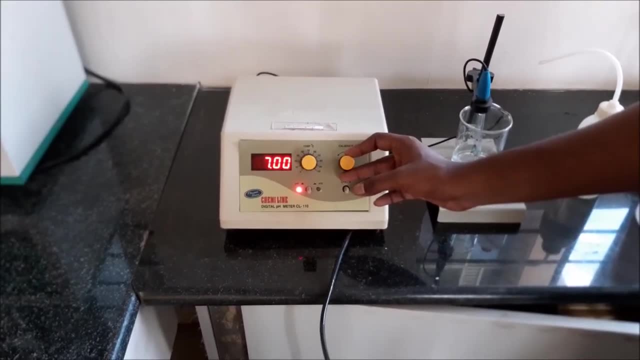 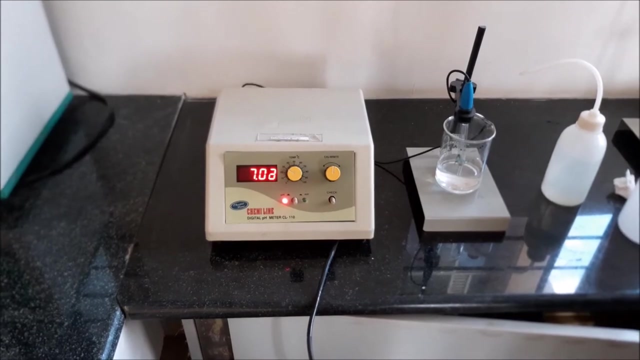 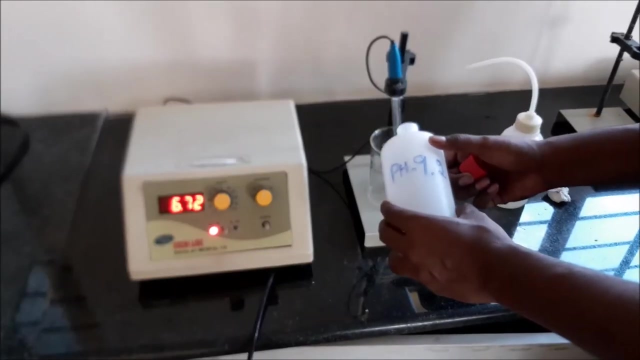 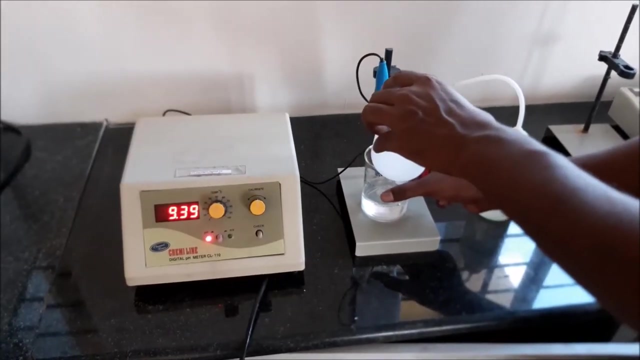 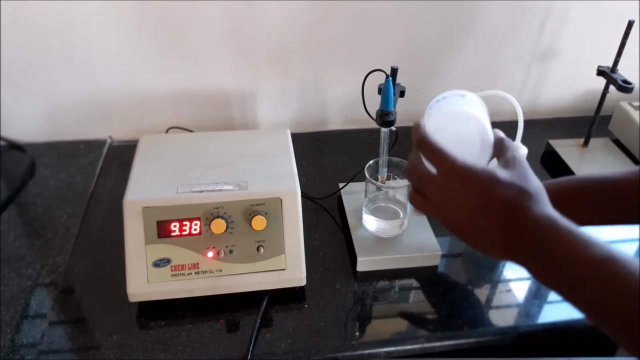 to calibrate the ph value equal to 7, the knob is adjusted so that the ph value is almost equal to 7.. Now the calibration is completed. The next set of buffer solution for the calibration of pH value equal to 9.2 is taken in the beaker. 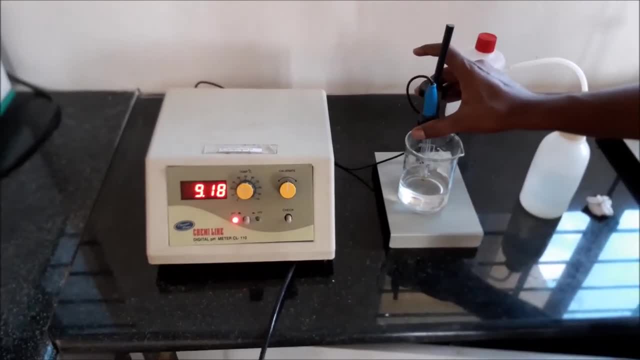 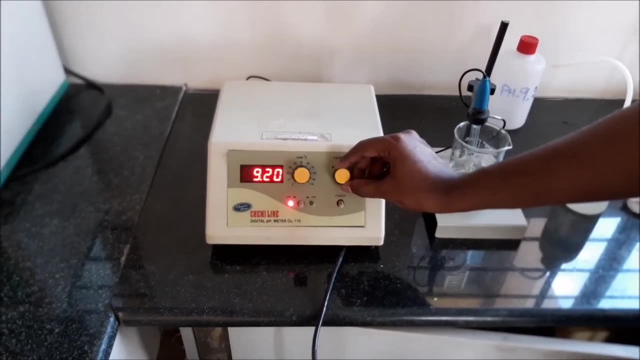 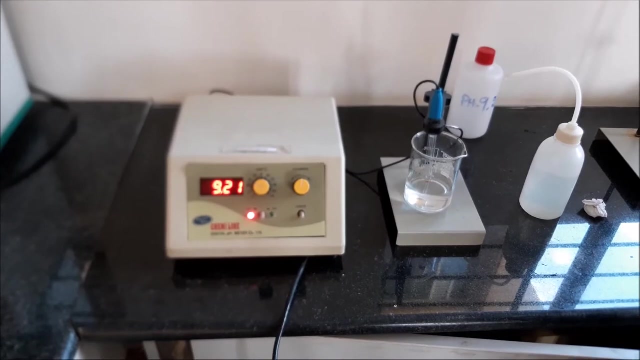 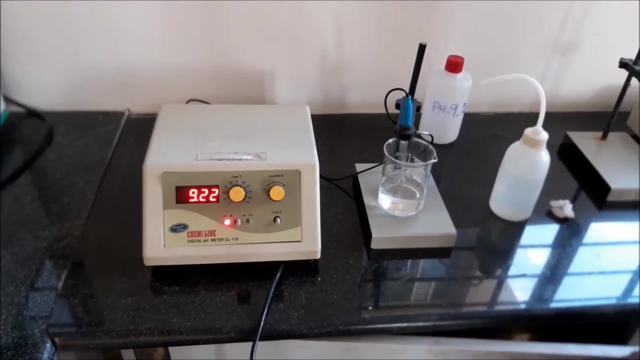 and then the electrode is immersed into the buffer solution to make sure the value is almost equal to 9.2. We can adjust the knob to wait for couple of seconds so that, like the pH value is calibrated to value equal to 9.2.. So this completes the calibration. 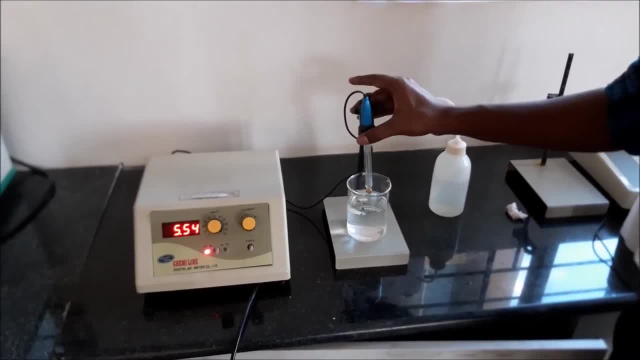 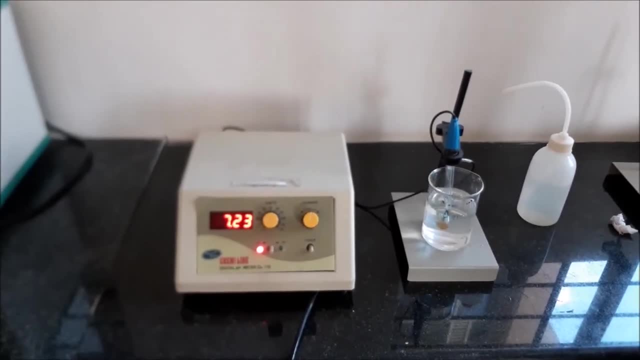 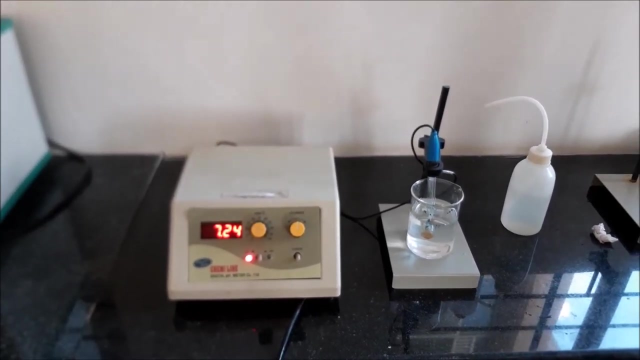 part. The tap water is taken in a beaker and the electrode is immersed and the pH value of the tap water is noted from the pH meter. A couple of seconds is needed to be waited and then the reading is to be noted. The reading: 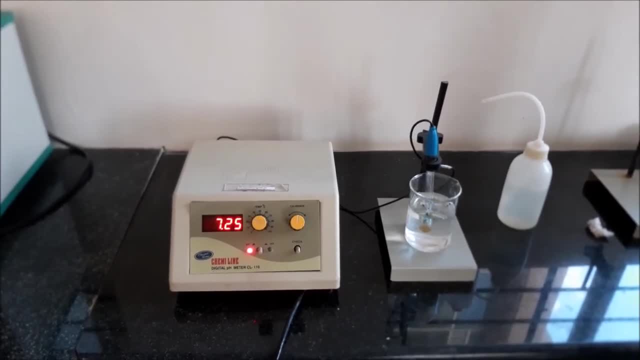 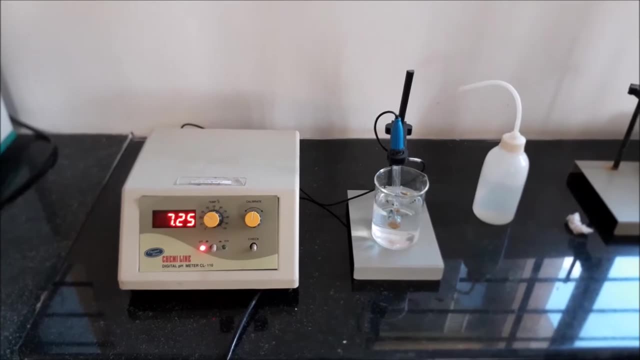 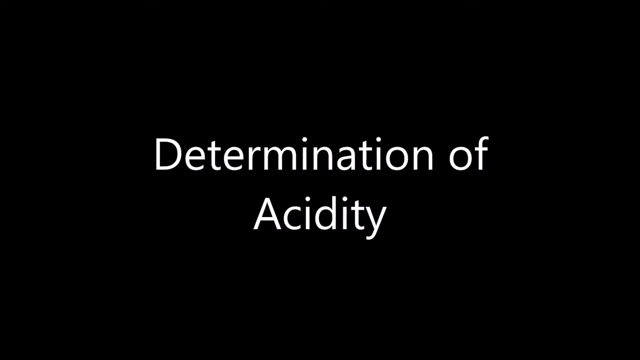 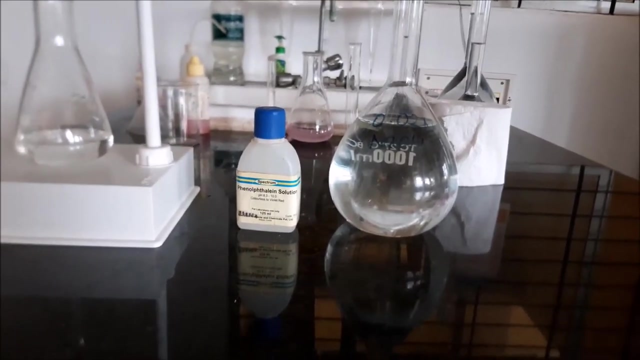 is 7.24 approximately. Since the pH value is more than 7,, the tap water sample is considered to be alkaline. As you can see here, today we are testing for total acidity, So we have taken 0.02 normality. 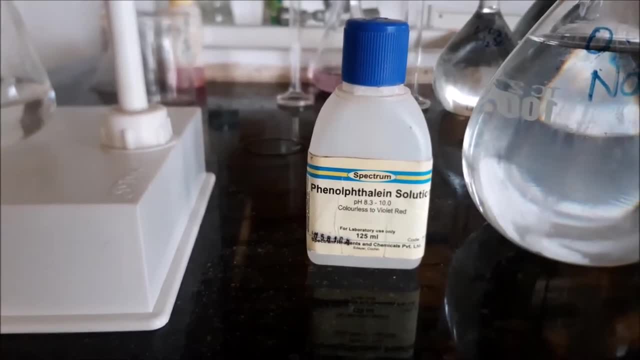 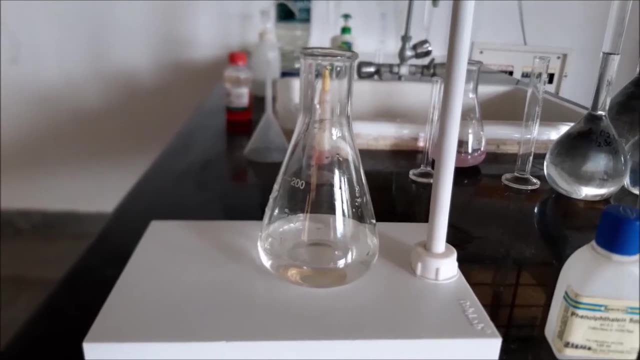 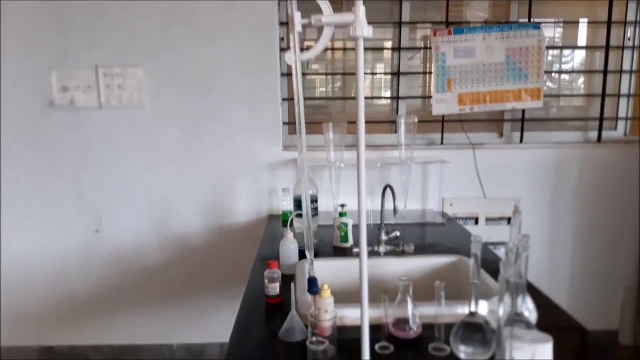 of NaOH solution. We have taken phenolphthalein indicator and in the conical flask we have taken the sample of domestic sewage water. a 50 ml of sample is taken here and in the burette This is filled with 0.02 normal of NaOH. So now we are adding the indicator to the sample. 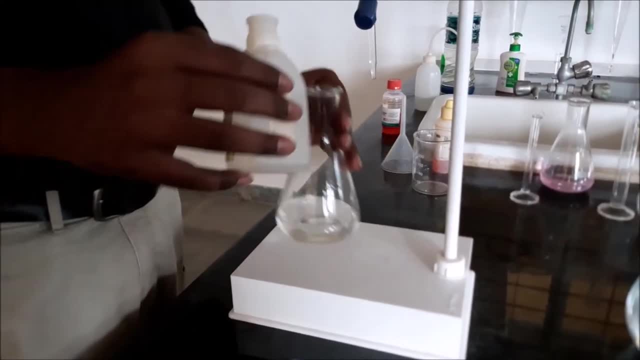 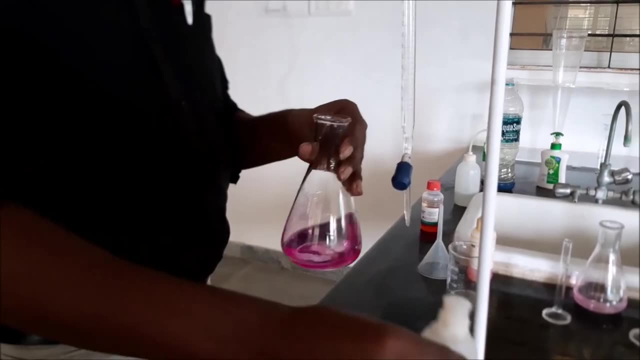 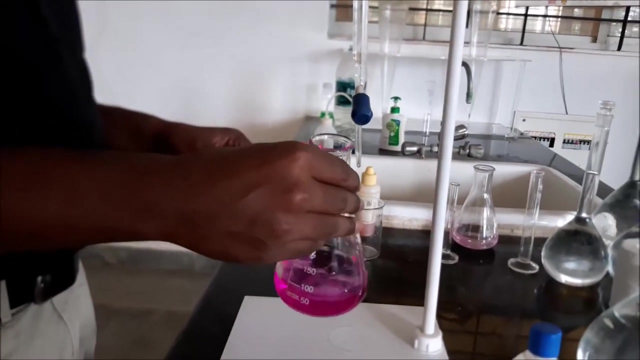 A few drops of phenolphthalein indicator is being added to the sample. As you can see carefully, just on adding a drop of phenolphthalein indicator, the colour has changed to permanent pink colour. So this indicates that upon adding the phenolphthalein indicator, if the 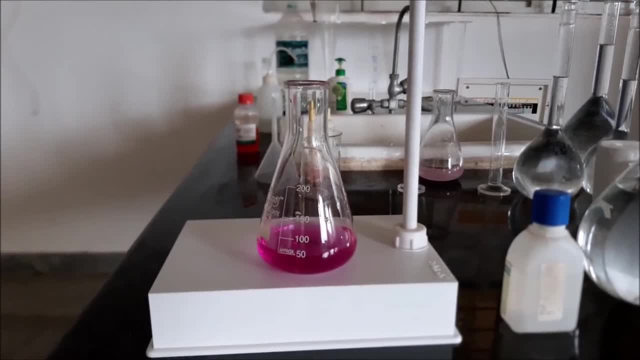 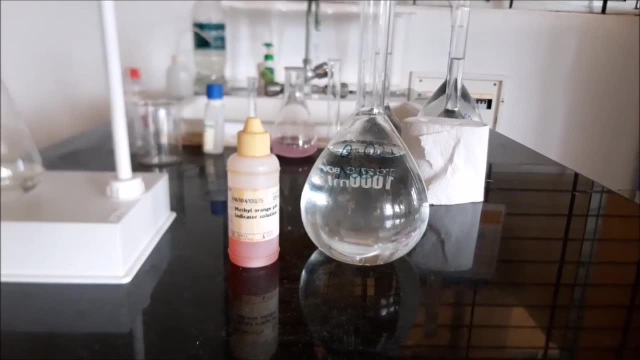 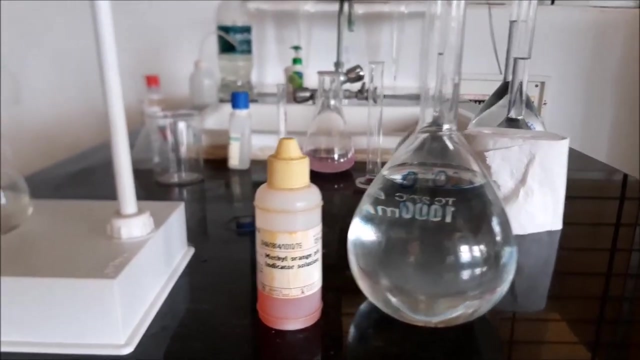 colour is changing to pink colour, it means total acidity is absent in the sample and there is no need of titrating it. As you can see, here today we are checking for mineral acidity. So we have taken 0.02 normality of NaOH solution, We have taken methyl orange indicator and in the conical 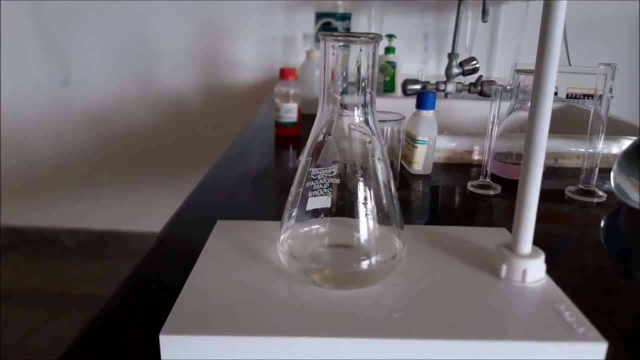 flask we have taken 50 ml of domestic sewage water. in the sample and in the burette we have filled 0.02. normal NaOH solution is taken. We can control the buried salt content anyways. Thus, after clue theuni said water amount of Pardon: 10 sterling is наша remission覺得. 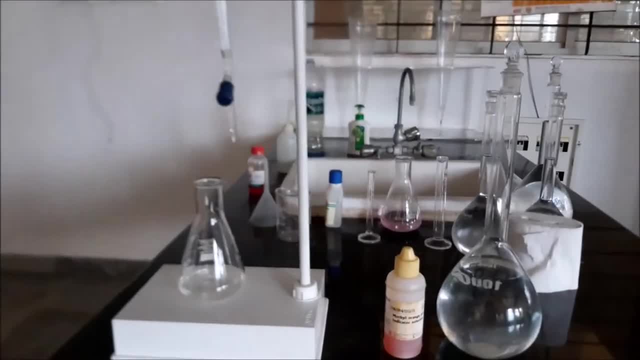 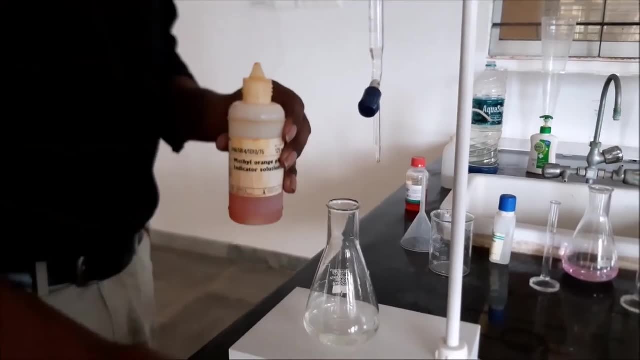 insecure about soufflier Because of bad water quality of a云ychgh bureti rohe Elektratoy scriptures. So for the sample now let us add methyl orange indicator. so a few drops of methyl orange indicator is being added to the sample. 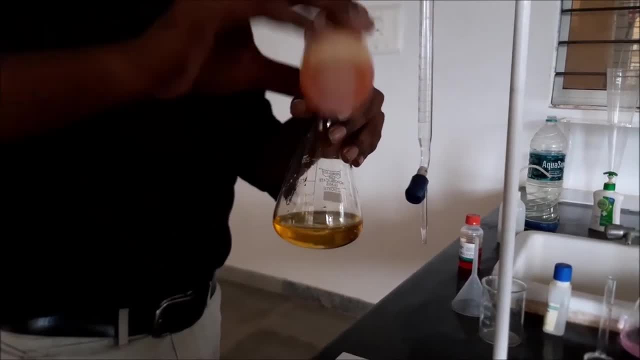 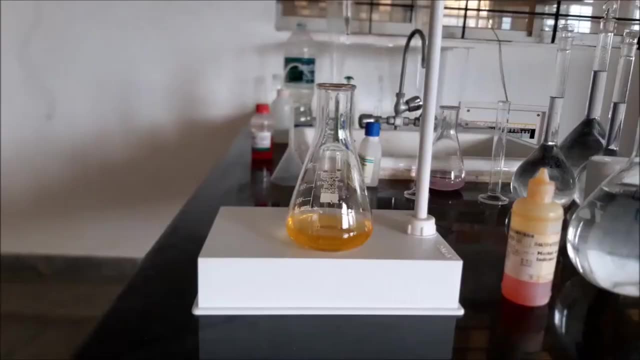 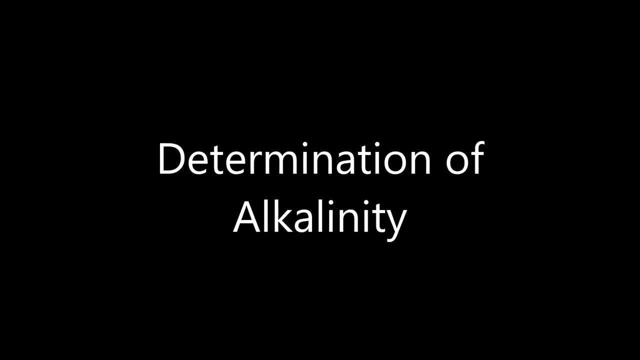 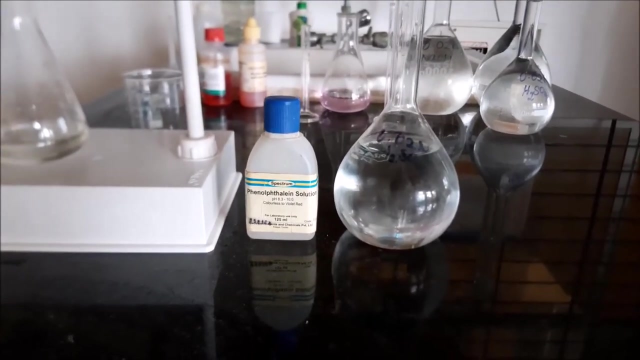 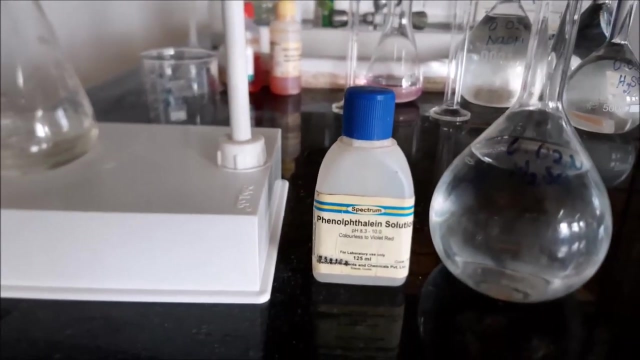 As you can see, see, upon adding the methyl orange indicator, the sample has turned to yellow color, which indicates that mineral acidity is absent. so no need of titrating it. So today we are checking for phenolphthalein alkalinity. So for phenolphthalein alkalinity we have taken 0.02 normal H2SO4 and the indicator. 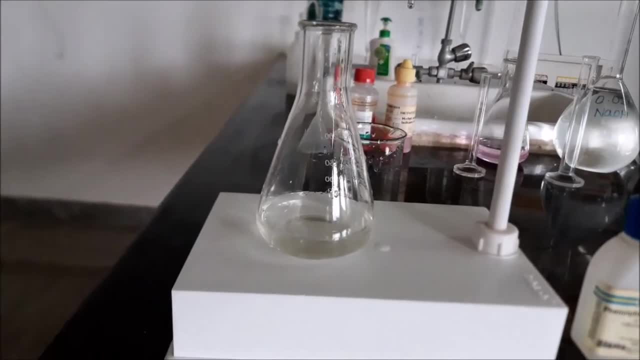 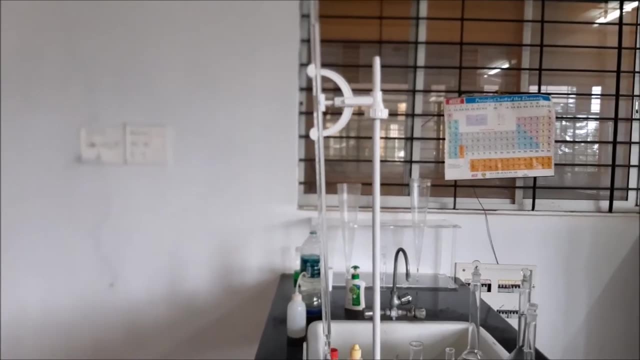 is phenolphthalein indicator and in the conical flask we have taken 50 ml of sewage water and again in the burette we have filled 0.02 normal of H2SO4.. So now for the sample. we are adding the phenolphthalein indicator. 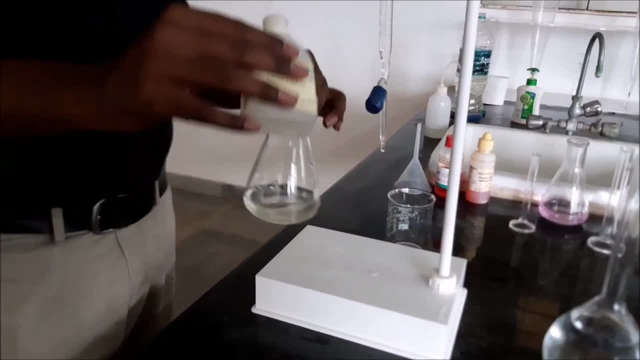 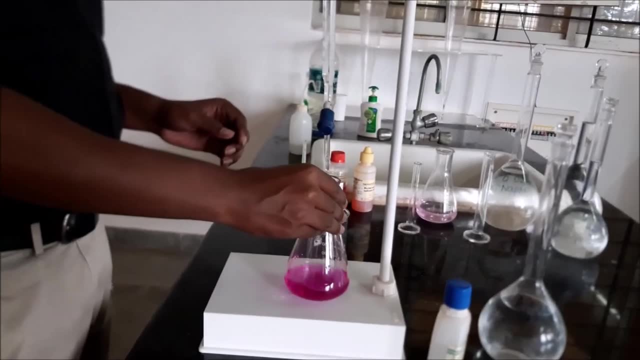 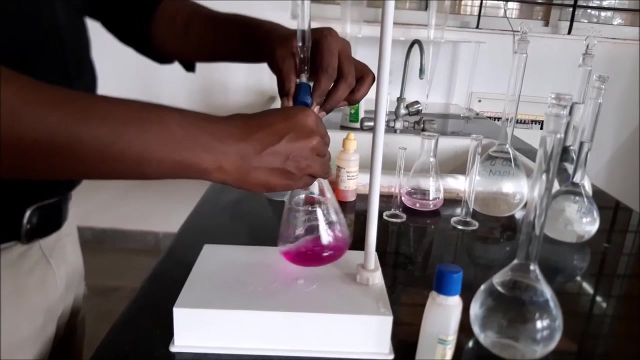 Phenolphthalein indicator is being added, it changes to pink color, which shows that the alkalinity is present. so we have to titrate it again as 0.02 normal H2SO4.. So initial rating of the burette is 0. as we are titrating it it changes from pink color. 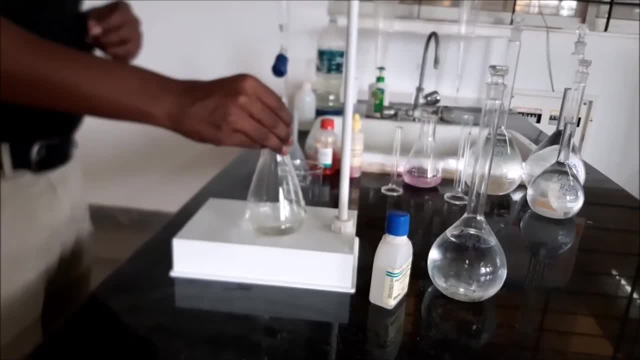 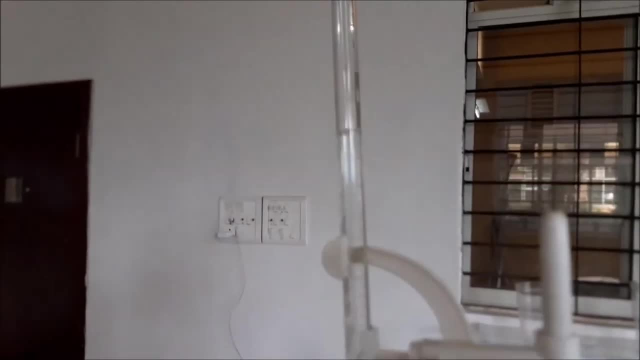 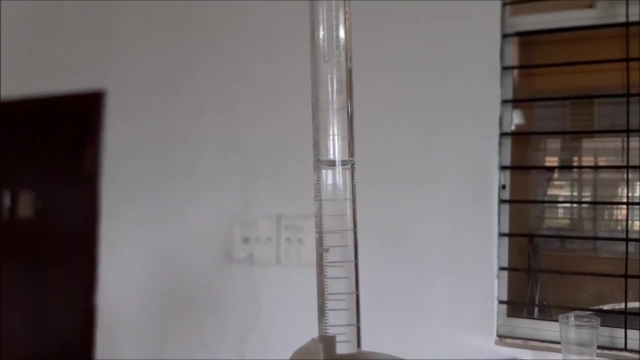 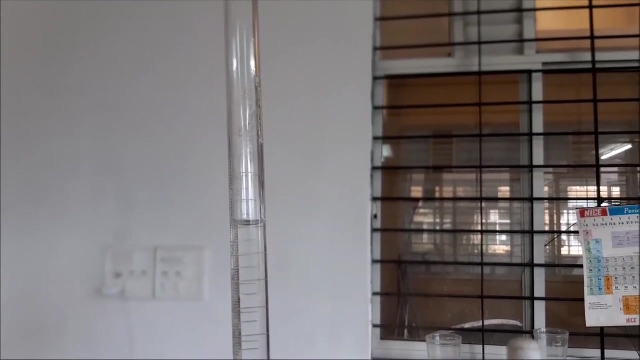 to permanent colorless, which shows that naphthalene alkalinity is present. and now you have to note down the final burette rating, which almost comes up to 0.8.. Note down the burette rating. The burette rating noted down is being used for the calculation of total alkalinity using 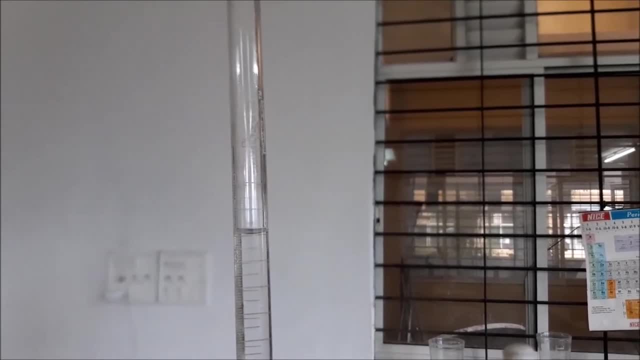 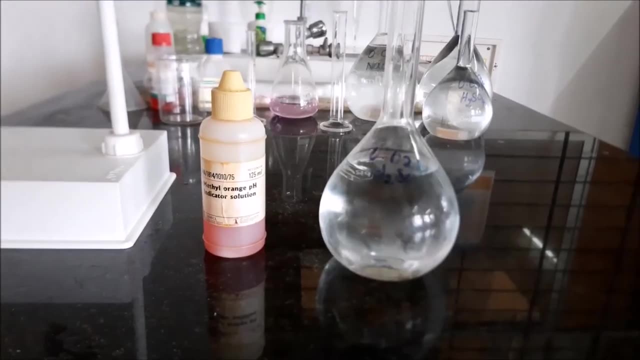 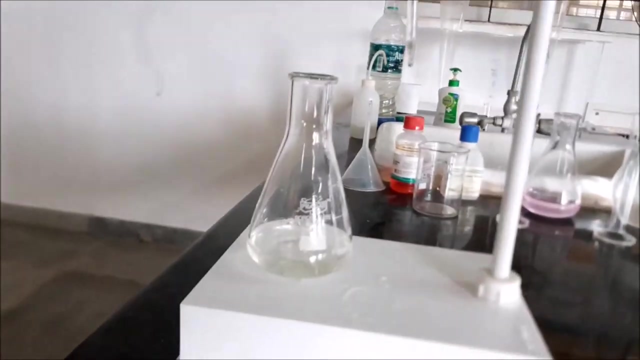 the formula given in the lab manual. So today we are testing for the total alkalinity. We have taken 0.02 normal H2SO4.. We have taken 0.02 normal H2SO4. And the indicator here is methyl orange indicator. and in the conical flask we have taken 50 ml. 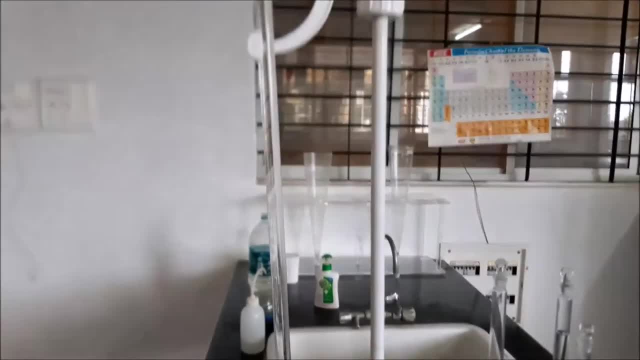 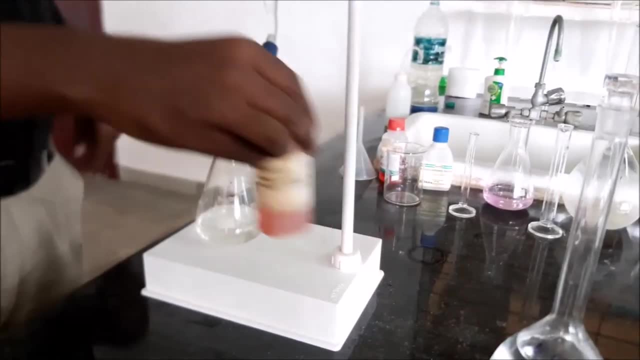 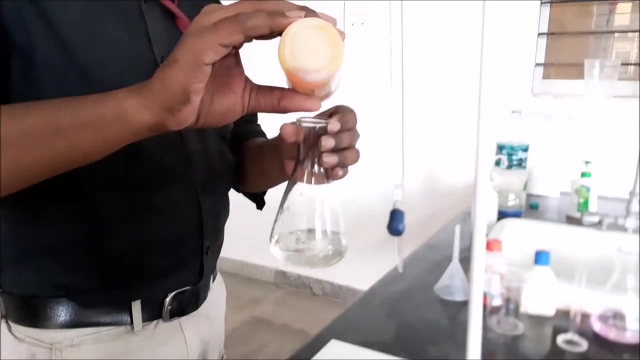 of sewage water and in the burette we have filled it with 0.02 normal H2SO4.. Now the indicator methyl orange is being added to the sample. As you can observe, 1 to 2 drops of methyl orange is being added to the sample upon adding which.